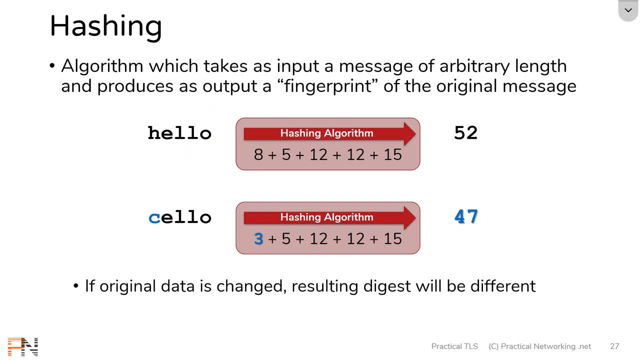 original messages are different. That's the purpose of a hashing algorithm. Now our hashing algorithm of simply adding up the letter values works as an example, but it's a pretty poor actual hashing algorithm because there are obvious flaws to it In real life. 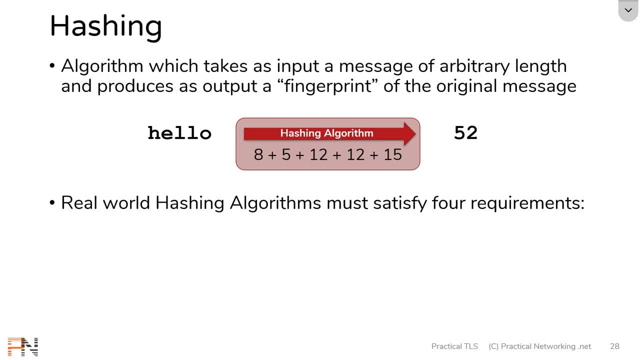 a hashing algorithm is approved for daily use, There are four requirements that that hashing algorithm has to meet. The first of those requirements is that the hashing algorithm must make it infeasible to produce a given digest. If I challenged you and said how many? 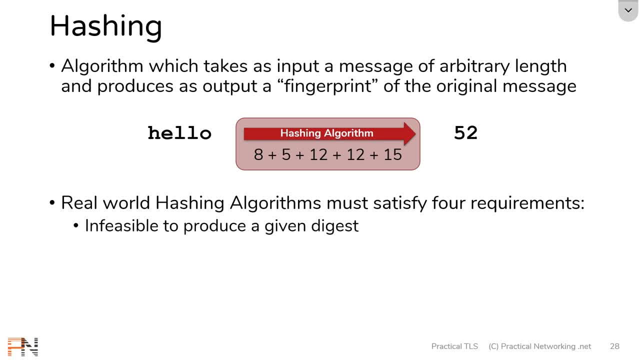 words can you create that add up to 52, it would just take you five to ten minutes to put together a list of words that add that up In a real hashing algorithm. that should be infeasible. It should be a task so difficult. it's borderline impossible. 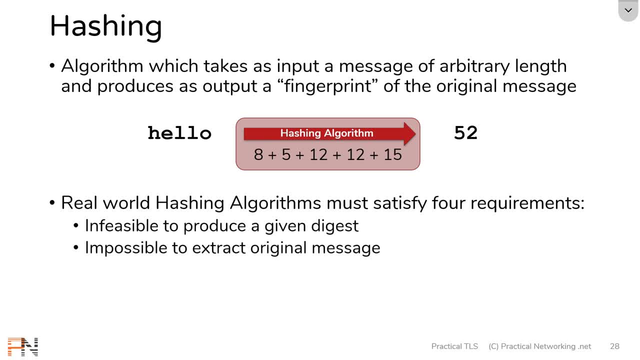 The next requirement is that the hashing algorithm must make it infeasible to produce a given digest. The next requirement for a real-world hashing algorithm is that it should be impossible to extract the original message. The idea is, if I give you a digest, it should be impossible to. 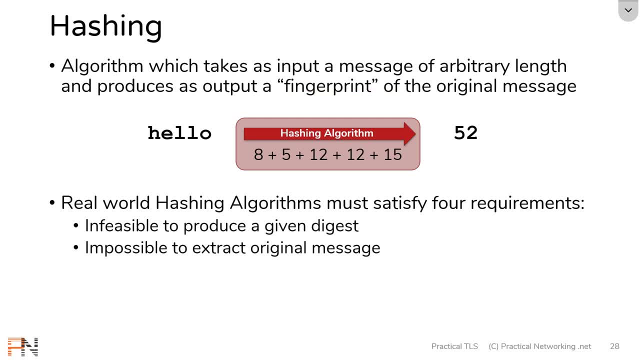 reverse engineer that back into the original message. In fact, hashing is sometimes referred to as one-way encryption. The idea is: you can encrypt something but you can never decrypt it. Technically, our letter addition algorithm does meet this requirement, because if I give you 52, there's no way for you to reverse engineer that back into hello. 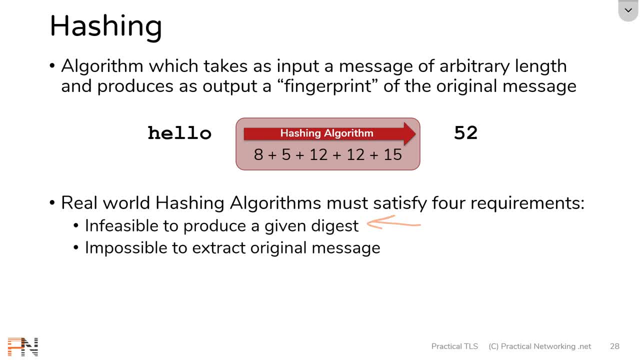 Maybe just because there could be so many different words that add up to 52. So technically, our weak algorithm does meet the second requirement. Either way, real hashing algorithms will definitely meet both of these requirements. The third requirement for a real world hashing algorithm is that 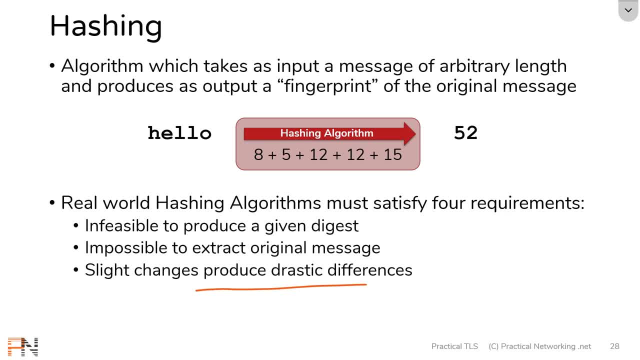 a small change to the original message is going to produce a drastic difference in the resulting digest. If I changed the word hello to cello, the resulting digest went from 52 to 44,. Well, that's a pretty small change. From that you can infer that the word cello is only a little different than the word hello. 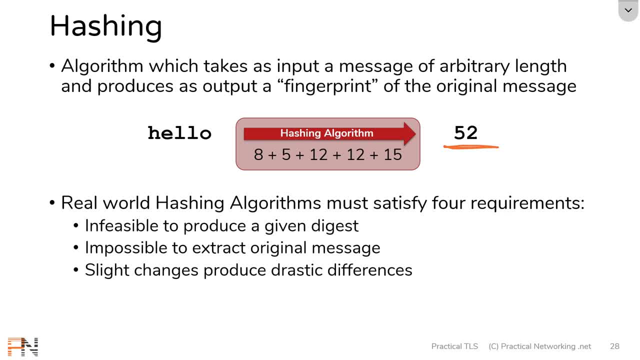 One of the ideas behind hashing is you want the resulting digest to provide zero hints as to what the original message was. Hence you want a small change to produce an unrecognizable difference. And the last requirement for a hashing algorithm is that the resulting digest must be fixed. 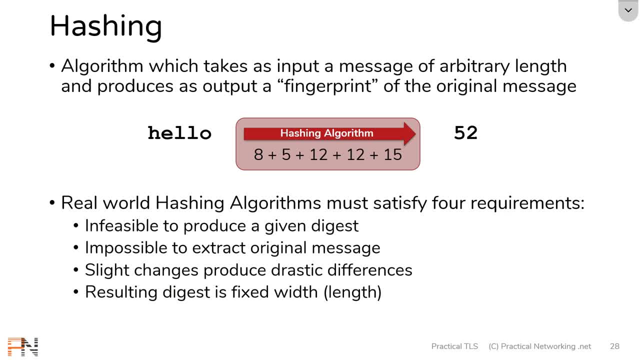 with, which is to say always produce the same length. digest. Here we hashed the word hello and got 52. If I hashed the string, how's it going? we would probably get a larger number. You can infer from the size of the digest of our algorithm the size of the original. 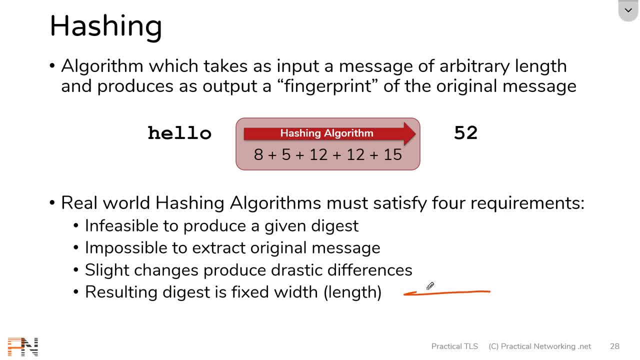 message that we hashed. That's bad. we don't want that. In a real-world hashing algorithm, whether you hash one letter, one word, one sentence or one entire book, the resulting digest is always the same length. Now I want to prove each of these things to you. 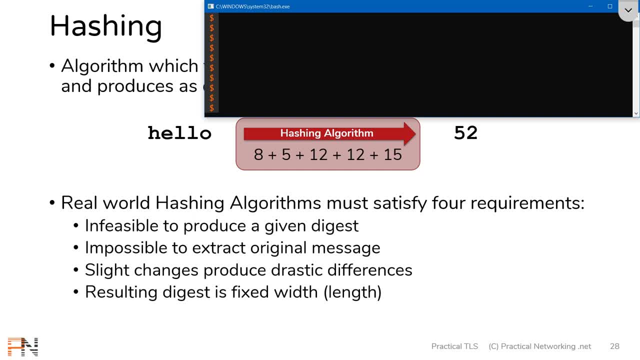 This is a bash terminal. I'm simply using a version of Ubuntu running on a Windows box, but what I'm about to show you can be done with any Linux distribution, so you're welcome to follow along. Most Linux distributions have the echo utility. 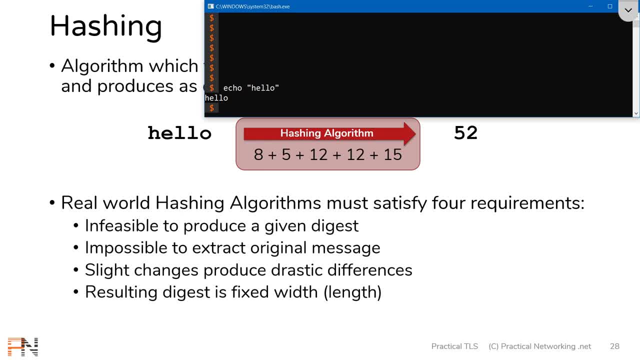 The echo utility lets you send something to standard output. I also have the ability to redirect what I just sent to another Linux utility known as the MD5.. The MD5 sub-utility is going to calculate the MD5 algorithm on what I send to it. 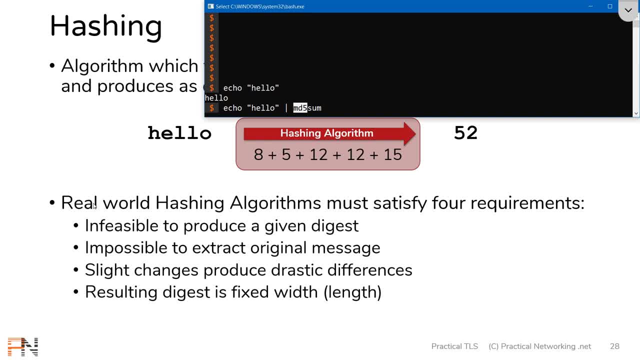 MD5 is a real-world hashing algorithm, so it's going to match these four requirements. If I hit enter here, you'll see that this is the result of sending the string hello through the MD5 algorithm. If you're following along, you should have got the same thing if you hashed this exact. 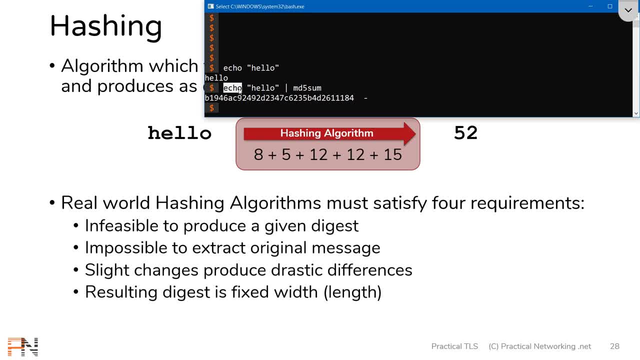 same message. Now I should mention that the echo utility automatically adds a string to the string. It automatically adds a newline character at the end of what is echoed. If you wanted to avoid that, you can prefix the echo utility with the argument "-end". 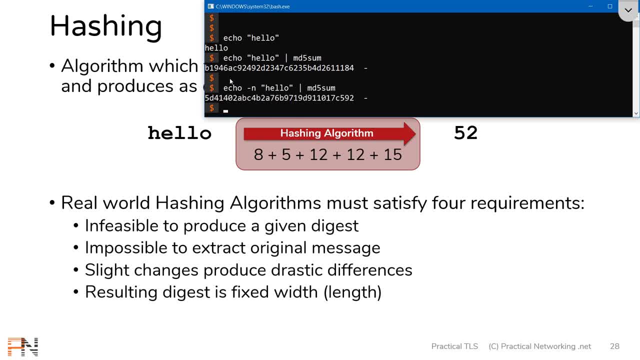 So, either way, whatever hashing algorithm or program you use, if it's doing MD5, if you run the string hello with a newline character, you'll get this, or hello without a newline character, you'll get this. Anybody doing MD5 on this exact same message- in this case, the word hello will always get. 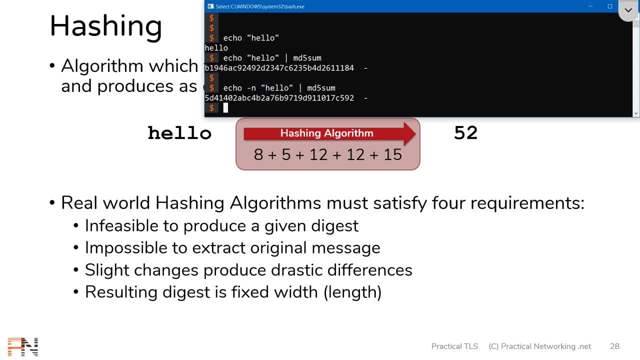 this result. Now let's talk about these requirements down here. This first one says it should be infeasible to produce a given digest. If I sat you in a room with a computer, could you create a bunch of messages that add up? 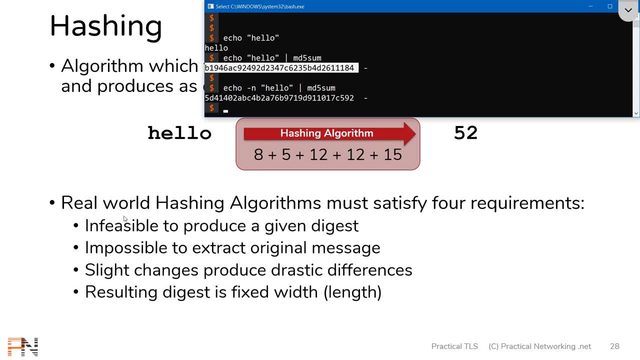 to that same result? Probably not. In fact, it's very, very difficult, Borderline impossible. That's what this first requirement is. Moreover, this second requirement: impossible to extract the original message. could you take from this and reverse engineer this back into the string? hello. 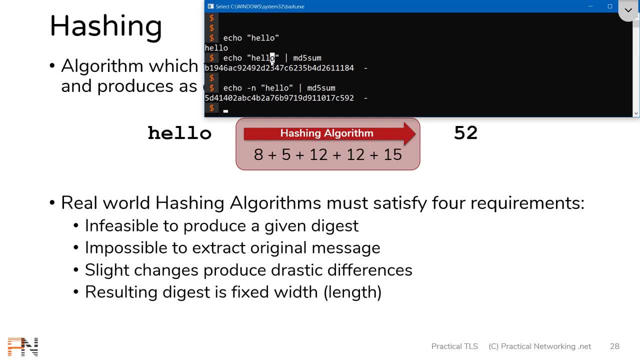 You can't, It's actually impossible. Now for this next one. I'm going to create a longer hash. I'm going to go ahead and echo the string. the quick brown fox jumped over the lazy dog to the MD5 utility. Notice whether I hashed five letters, rather five letters with a newline character five. 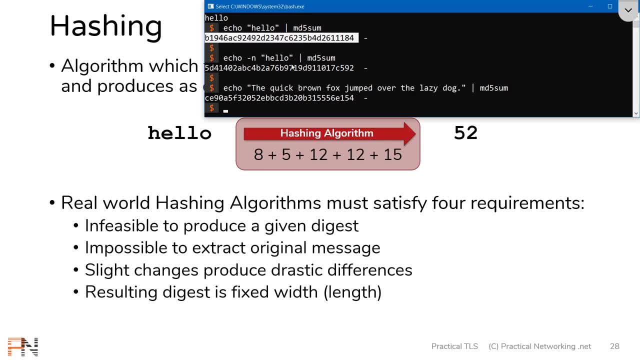 letters by themselves or a whole sentence. no matter what, the resulting digest was still the same. That's actually kind of an example of this last one. The resulting digest is fixed width. Now, if I take this last sentence and I make a very small change, let's just capitalize. 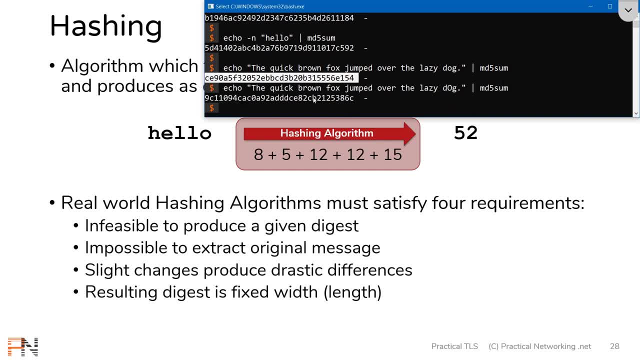 this letter in the middle of the word dog, you'll notice the resulting digest is extremely different. That's this slight change produced drastic differences. Now, internally, the way that works is. a hashing algorithm is not simply one calculation done on the original message. 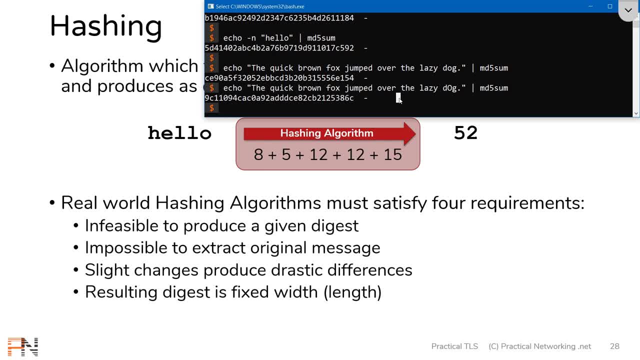 It's actually a calculation done and then iterated over and over and over to produce the final digest. So way in the beginning The difference might not be that big. But as it's continually iterated internally, the difference is going to get bigger and 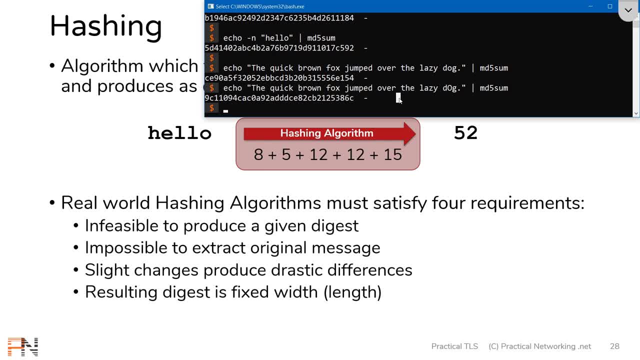 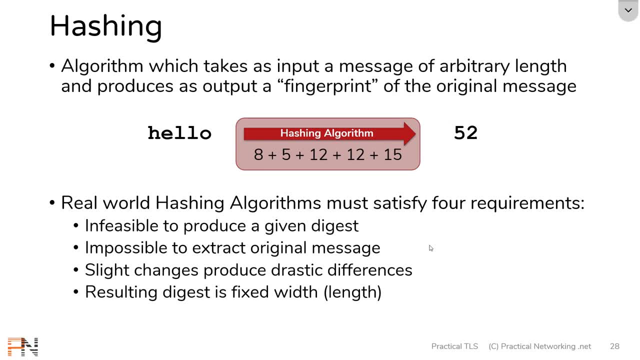 bigger to create that drastic difference. This effect is sometimes called the avalanche effect. Either way, hopefully, this proves the behavior that a hashing algorithm does and it proves these four requirements. So that's the definition of what a hashing algorithm is. Again, it's simply taking a message of arbitrary length and producing a message digest, which 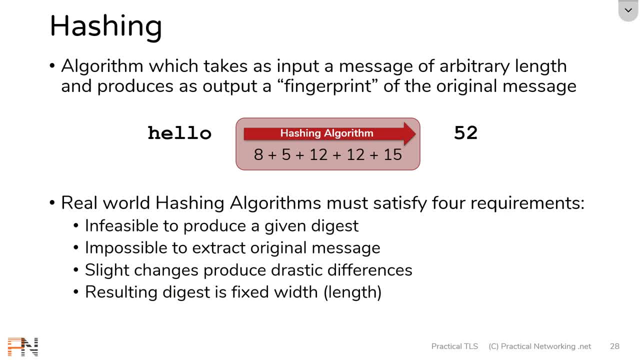 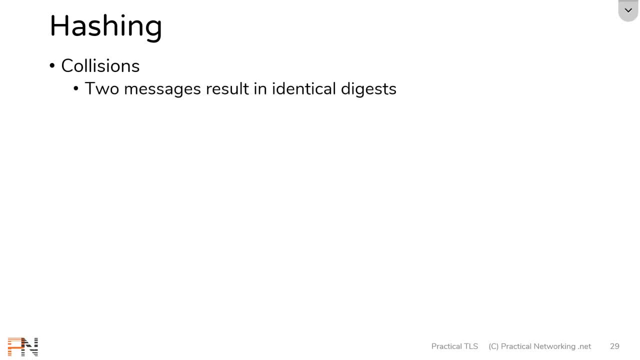 is unique to that particular message. Now, the last thing we need to discuss insofar as hashing is this idea of collisions. A collision occurs when two different messages add up to the same digest. This is a bad thing, because the purpose of hashing is to compare two messages to see. 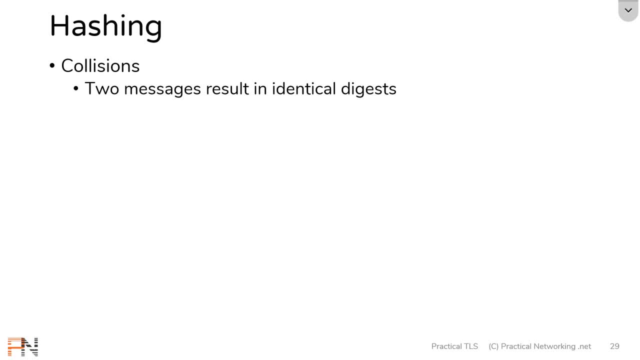 if they're the same or they're different. Well, if there are two messages that add up to the same digest, then you're never going to be able to tell them apart using a hashing algorithm. So collisions are a bad thing. The problem: 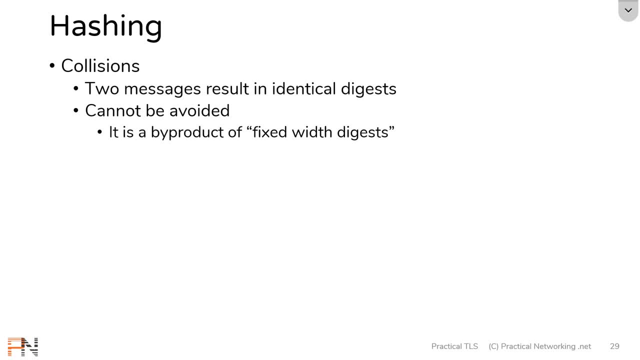 However, Collisions are unavoidable. It's actually simply a byproduct of the idea of fixed width digests. So let me explain that. Let's make up a new made up, imaginary hashing algorithm. We're going to call it the prac hash. 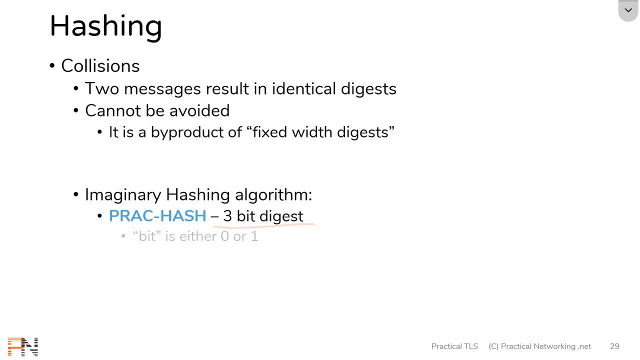 The prac hash is going to create a three bit digest What that means. a single bit can be a zero or a one. If I have three of them, that means I have three positions that can each either be zero or one. If we map out every possible combination of three positions of the hash we're going to 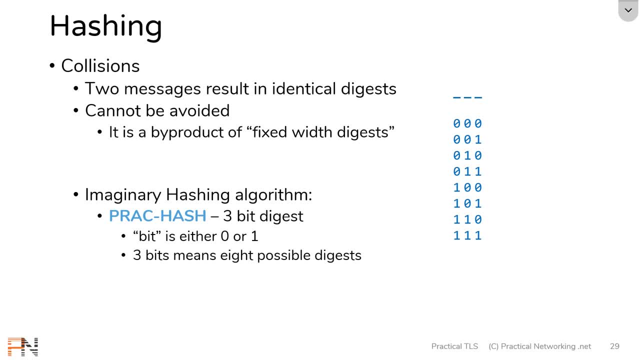 get zero or one, You would get this list that gives you eight possible combinations. Now you could also figure out that you have eight possible combinations by taking two and raising it to the third: two because there are two possibilities for each character- zero or one. and the third because this is a three bit digest that'll tell you we have eight. 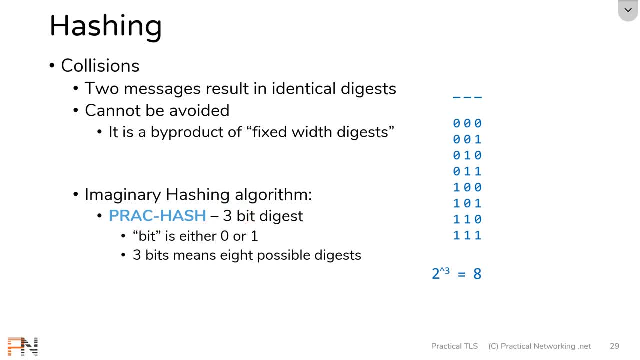 total combinations that the prac hash can put together. So if I were to run eight different messages through the prac hash, maybe that first one would map to that digest- Okay, And the second one would map to that digest, and the third one and fourth one and fifth. 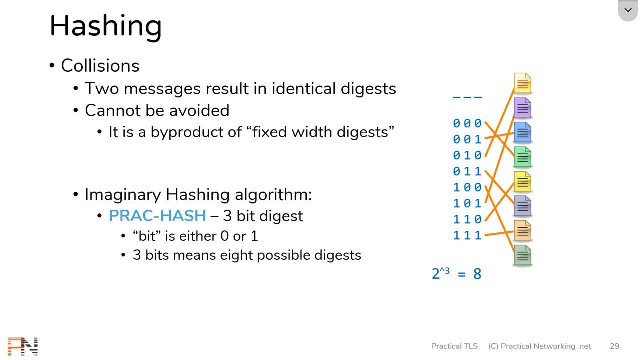 one Sooner or later. let's just say that all of them map to a unique digest going through the prac hash. Well, if, at that point, I decide to run a ninth message through the prac hash, no matter what the resulting digest is going to be, it's definitely going to end up mapping to a digest. 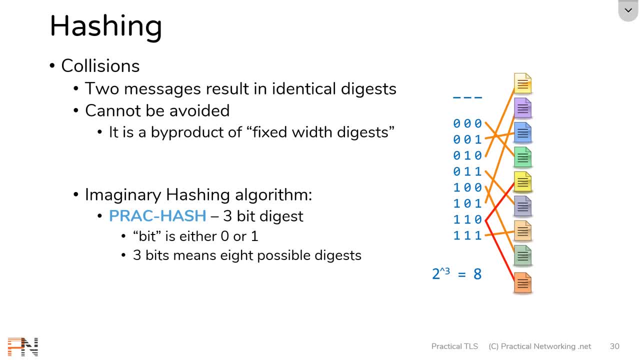 that another message already mapped to The simple fact that we only had eight possible digest that could exist and we ran nine message through them meant we definitely ran into a collision. That is what I was saying when I said that collisions cannot be avoided. 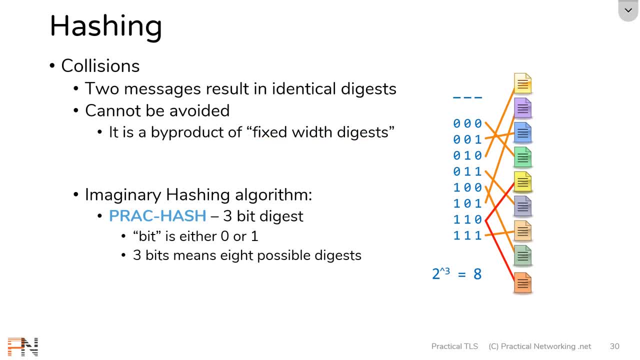 It's simply a byproduct of the fact that there are limited amount of possible digest for each hashing algorithm. Now they cannot be avoided. All you can really do is make them more rare. Generally, hashing algorithms that have a higher bit digest output are considered to. 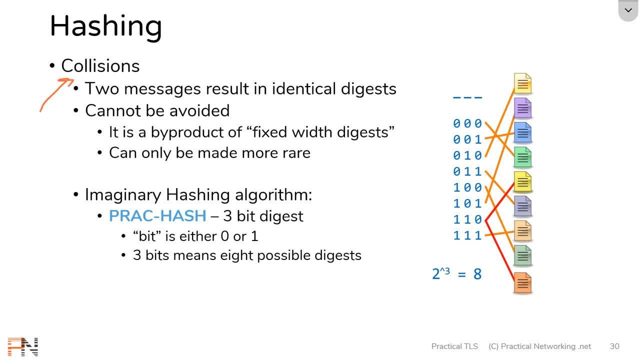 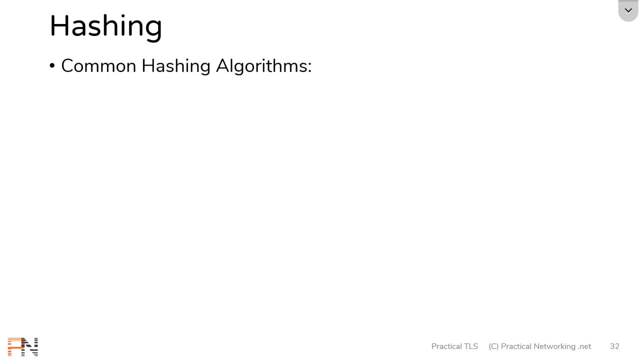 be more secure simply because they make collisions more rare. Finally, the last thing I want to show you is just a list of hashing algorithms that exist out there. We've already talked about MD5 just a little bit, but the two most common ones, you'll see.